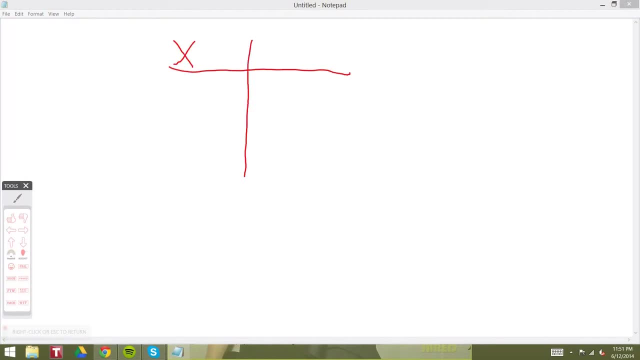 that sample is five data points, which are two, four, one, five and three. So the first step in this computational way is to take your X's and square each one of them, and when we do that we get 4,, 16,, 1,, 25, and 9.. So the next step is to 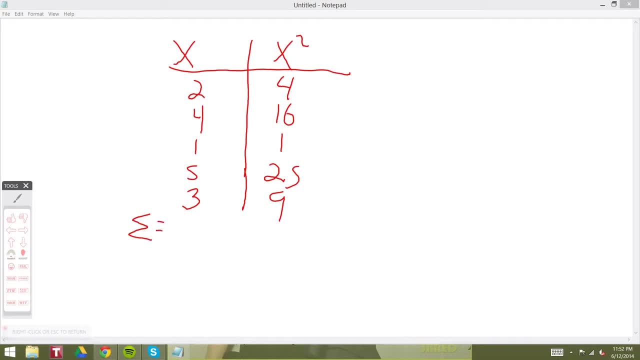 add up all of our X terms and all of our X squared terms and when we do that, we get 15 for the sum of our X squaresX values- sorry- and for our x squared terms we get 55, and once we do that, we are ready to solve for our ss. 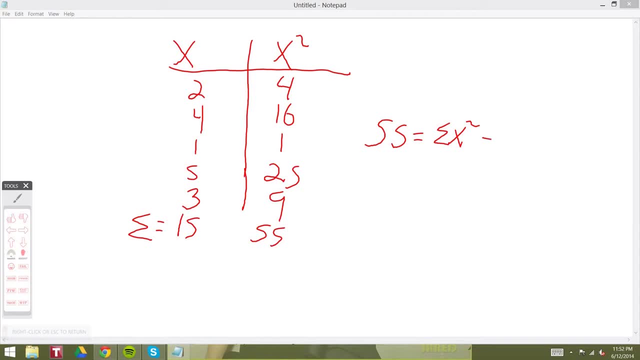 so we take our formula, which i will rewrite, and simply plug everything in. so we have 55 here minus a 15 here, and that is squared and that is divided by 5, because we have 5 data points in our sample. and when we do that, 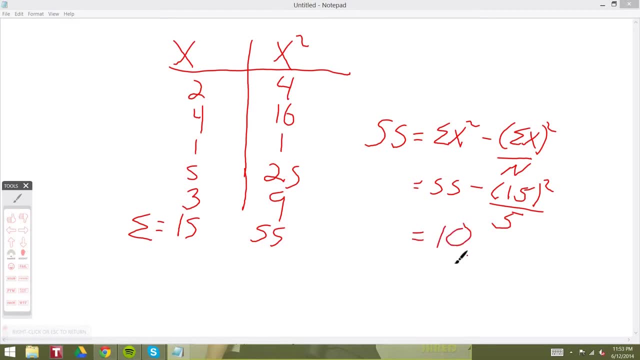 we get an ss v of 10 if you come. if you recall from the last video that when we found the SS of the sample using the definitional formula, we also got an SS value of 10. now that is not a coincidence and you will get the same SS value every single. 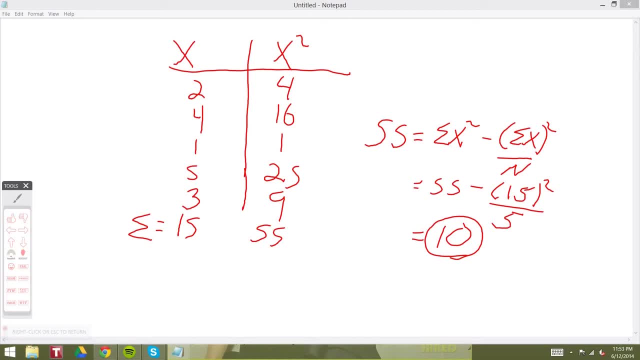 time, regardless of whether you use the definitional formula or the computational formula, so you can choose which one you want to use when you need to solve for the SS, whichever one you're more comfortable with. one advantage of this computational formula, however, is when you have a larger data set, whether 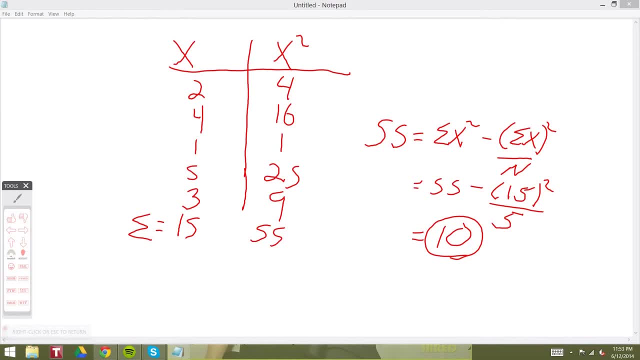 it be a larger sample or a larger population. so say, you have 20 data sets and you have 20 data sets, and you have 20 data sets and you have a sample of 20 data points instead of 5. it'd be much more tedious to go through.